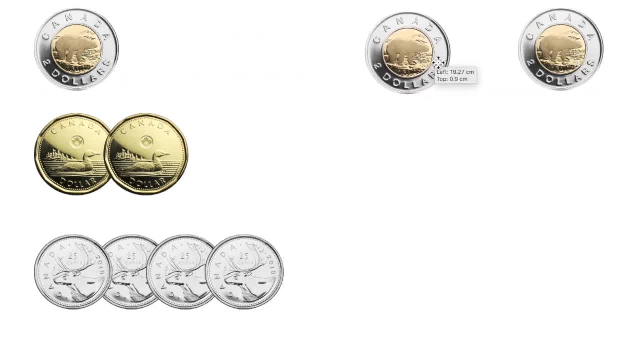 Two, four, six. Now we're going to move on to the next coin, which is step number three. We need to change our counting And we're adding on to what we've counted before. We were at six Toonies are worth $1.. Now we're counting by one, adding on to six. 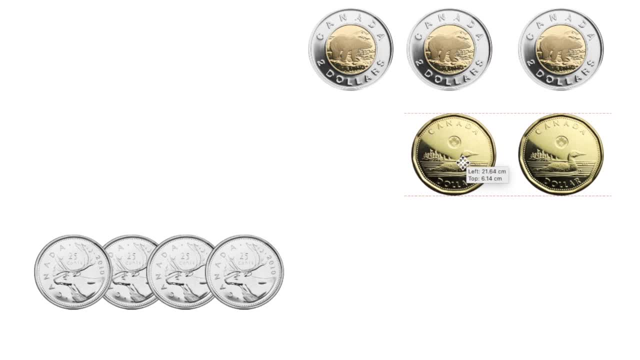 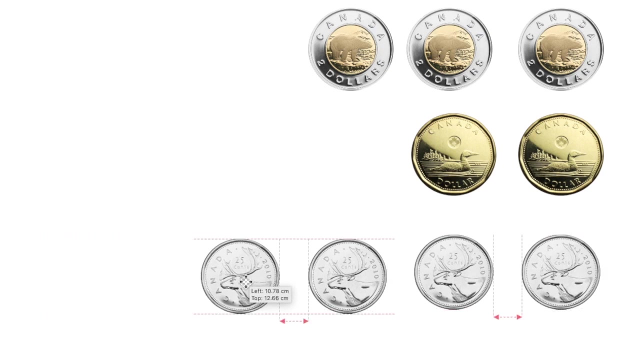 Seven, eight dollars. Now we're moving on to quarters. We are changing the way we count With quarters. we count by 25s And we're continuing with what we counted before, at eight dollars, Eight dollars and 25 cents. Eight dollars and 50 cents. Eight dollars and 75 cents Nine dollars, We have nine dollars. Let's count that again. 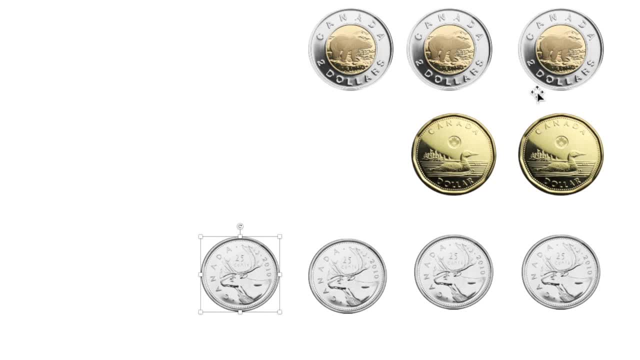 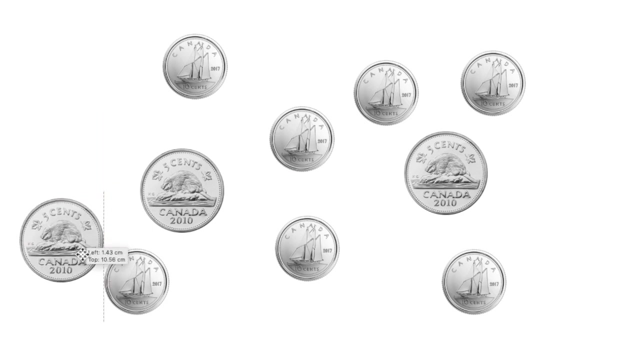 Two, four, six dollars. Seven, eight dollars, Eight dollars and 25 cents Eight dollars and 50 cents eight thousand seventy five cents nine dollars. let's try another one step. one: sort out the coins. we have dimes and we have nickels. 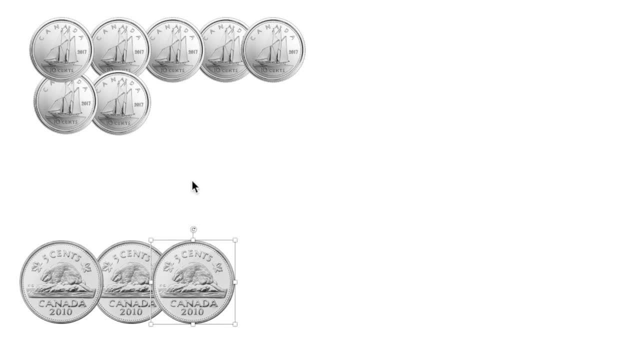 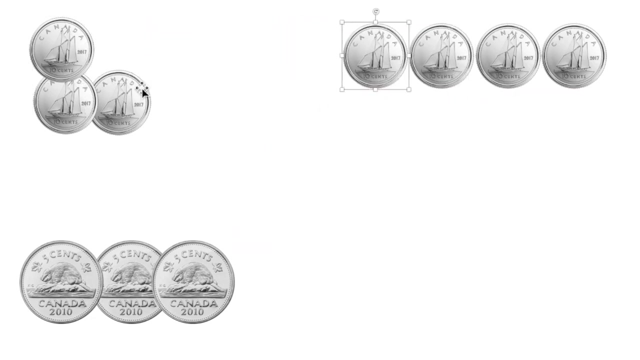 Dimes are worth ten cents and nickels are worth five cents. so we're going to start with counting our dimes. We're counting by tens: 10, 20, 30, 40, 50, 60, 70. Now we're counting our nickels. We need to change the way we count. 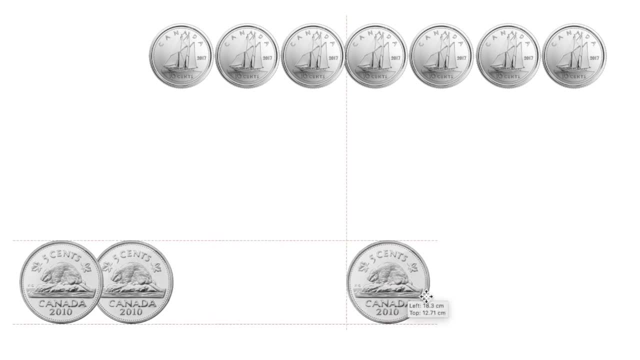 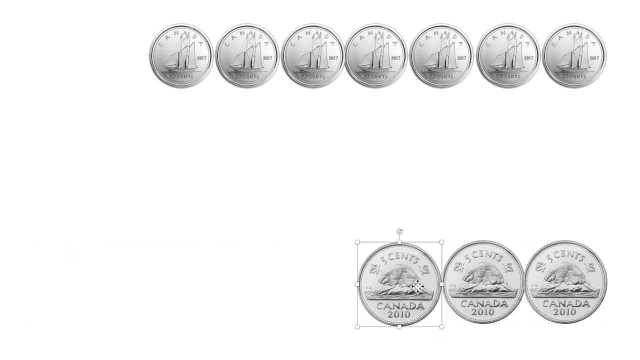 adding on to 70 cents, 75,, 80,, 85. We have 85 cents. Let's look at that again. 10 cents, 20, 30,, 40,, 50, 60, 70.. Change the way we count: 75,, 80,, 85.. 85 cents: Let's do one.